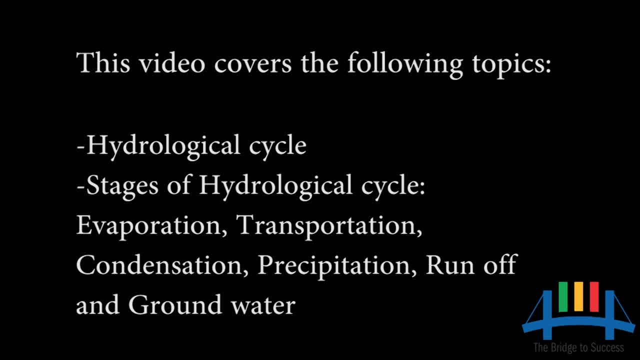 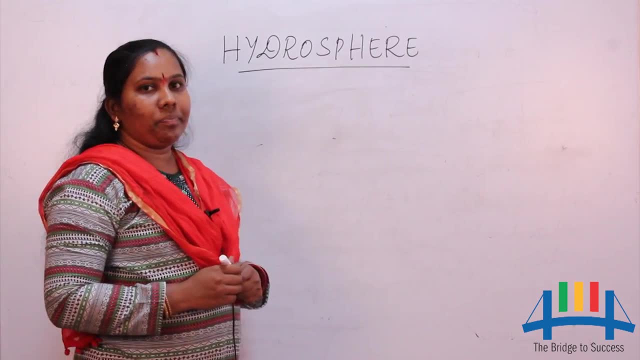 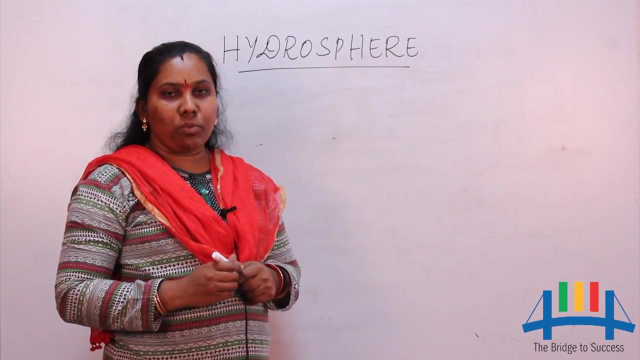 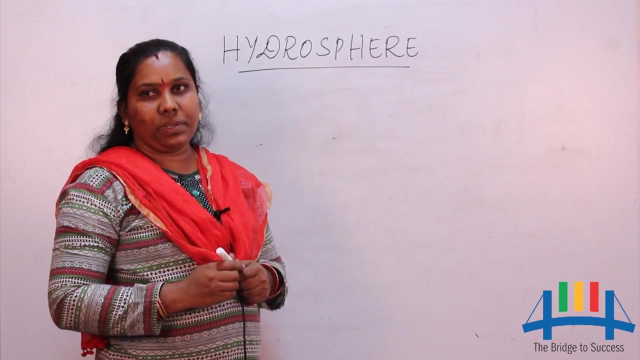 Hello friends. today's our topic is hydrosphere. As you have learned earlier, earth has four spheres: lithosphere, hydrosphere, atmosphere and biosphere. Today, we are going to learn about hydrosphere. Hydrosphere is the word which is derived from the Greek word. hydro means. 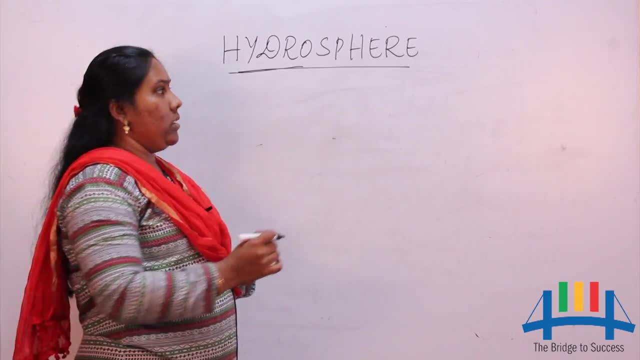 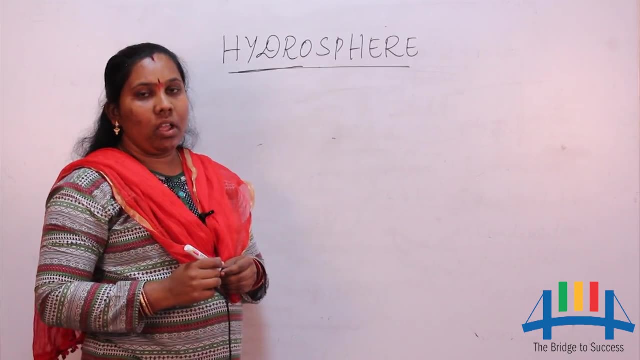 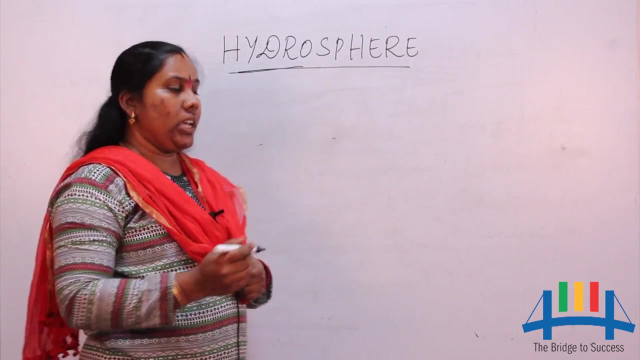 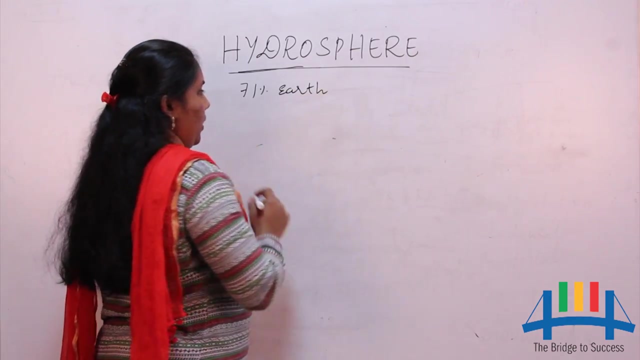 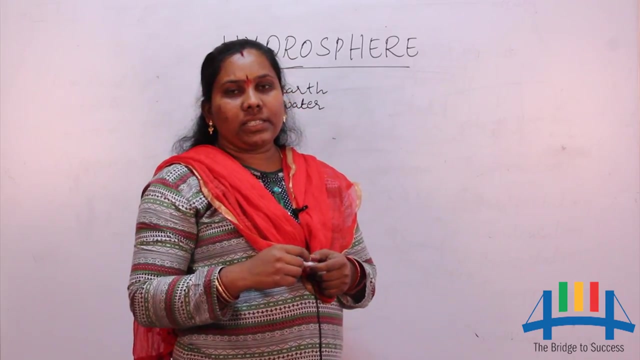 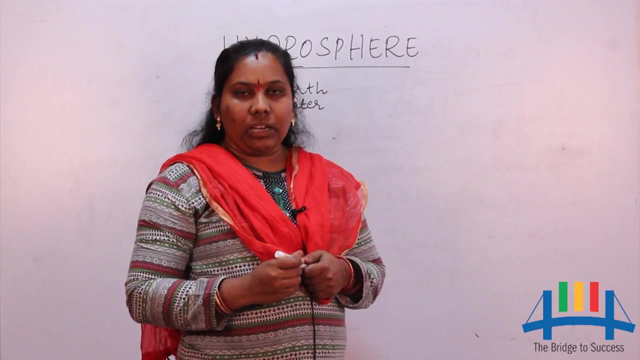 huder. huder, which means water. Spear is derived from the Greek word spheria, which means spear or a ball Water. without water, life cannot exist on the earth. Nearly 71 percent of the earth is covered by the water. Water is recyclable, renewable resource Because of water cycle. 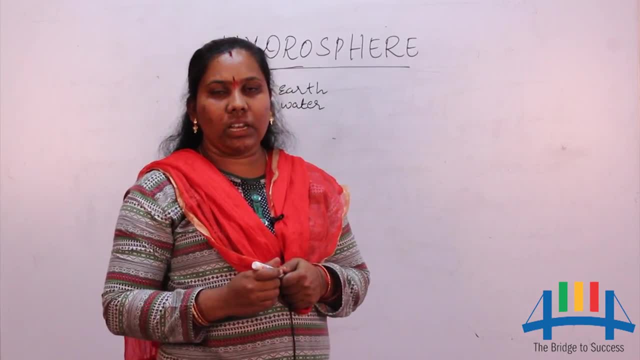 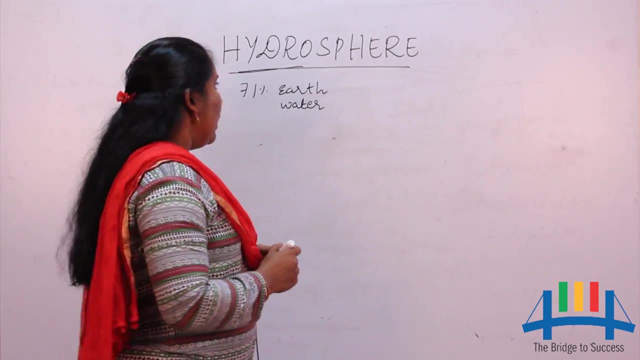 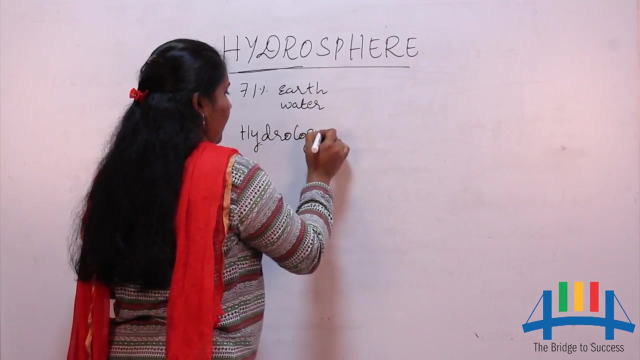 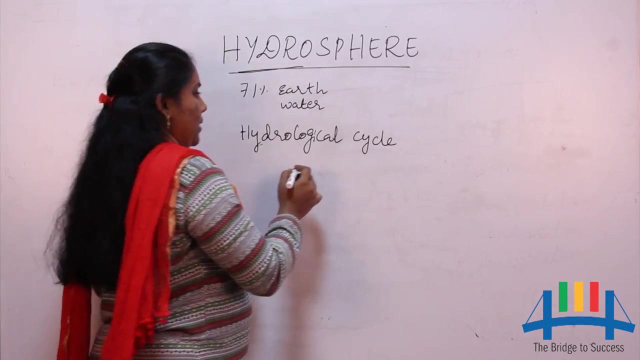 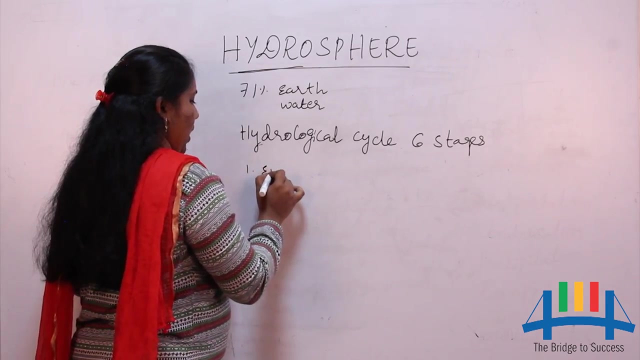 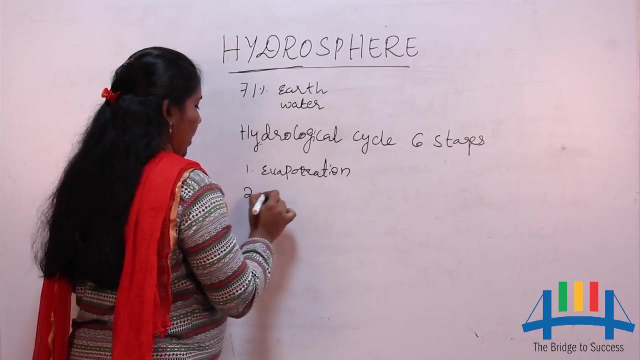 there are, life exists on the earth. This cycle is occurring from billions of years on the earth. Let us see what is this: Water cycle or hydrological cycle. Hydrological cycle has six stages. The first stage is evaporation. The second stage is transportation. 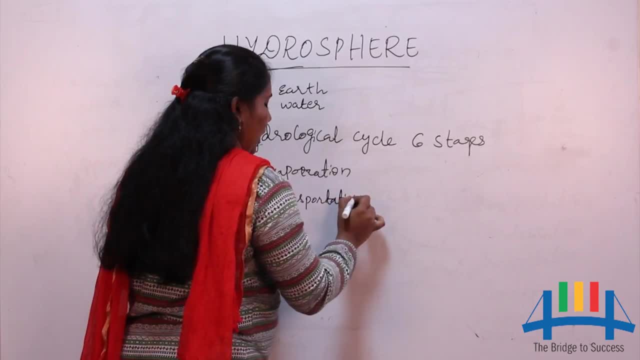 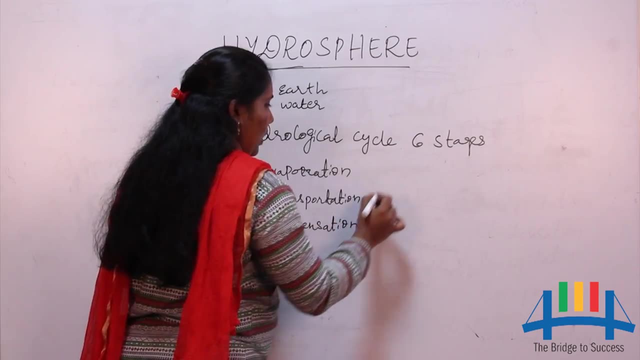 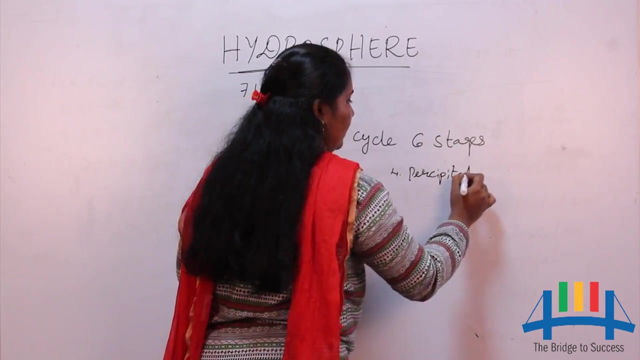 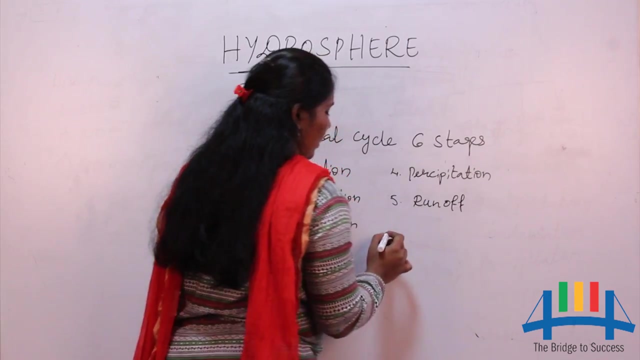 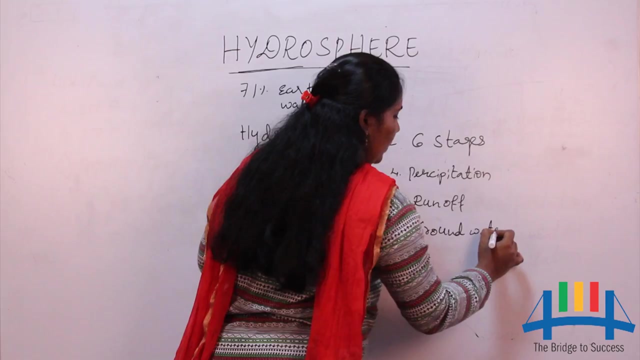 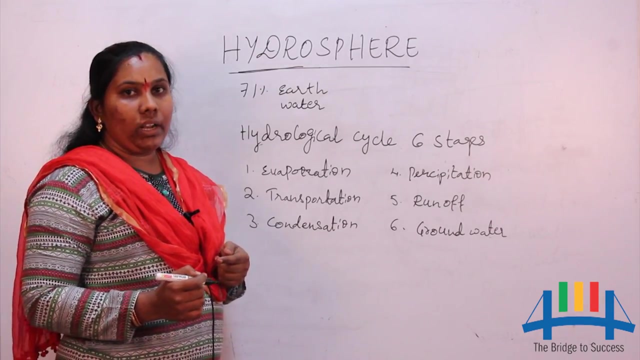 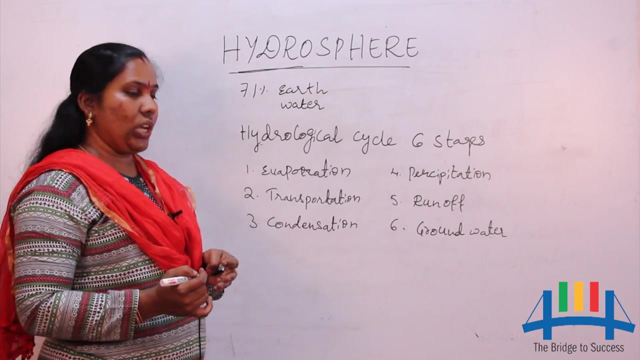 The third stage is condensation. The fourth stage is precipitation. The fifth stage is runoff. The sixth stage is ground Water. Let us see each one in detail. Evaporation: Evaporation is the process where the water is moving from the earth surface to the atmosphere, that is, from the liquid form it is changing into. 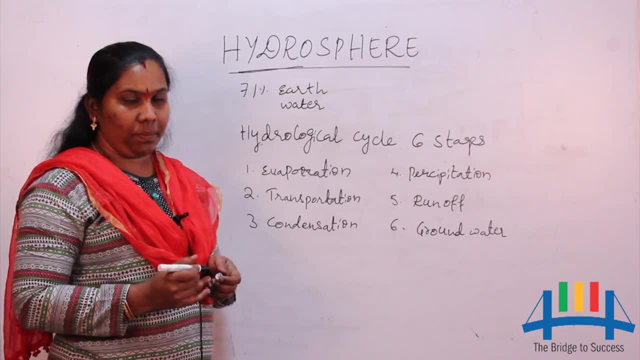 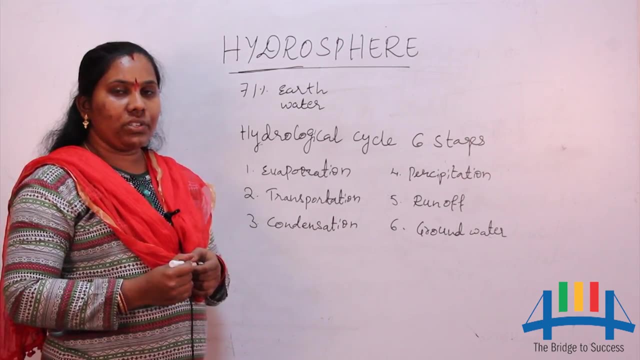 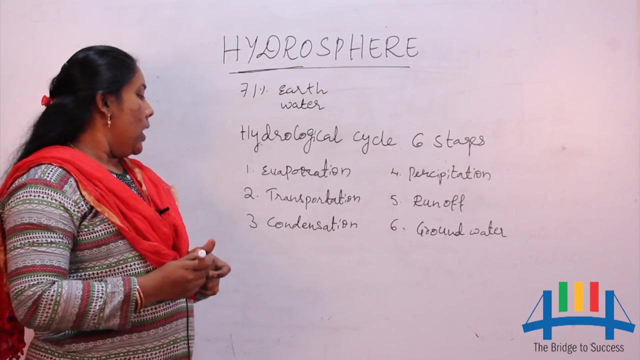 gaseous form, which we call as the water vapor. Evaporation occurs from the water surface, like oceans, seas, rivers, lakes, as well as from the planet. This is called evapotranspiration. The second stage is transportation: The water which has moved. 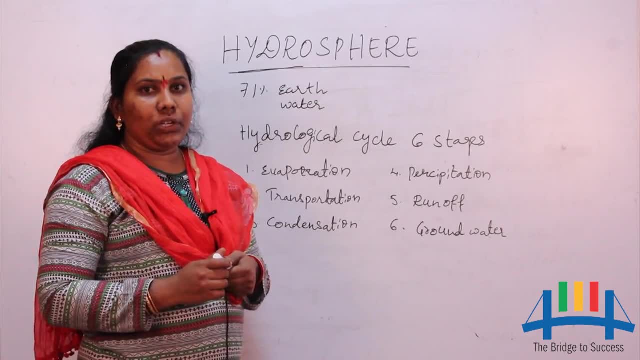 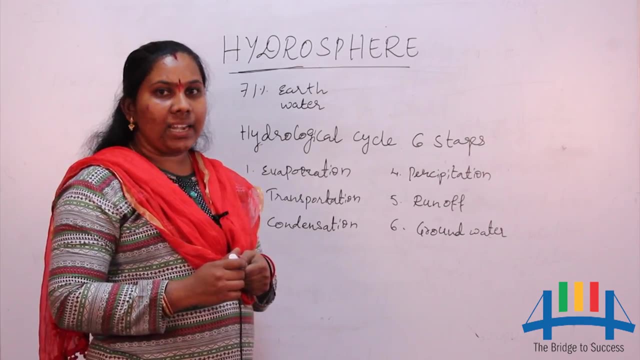 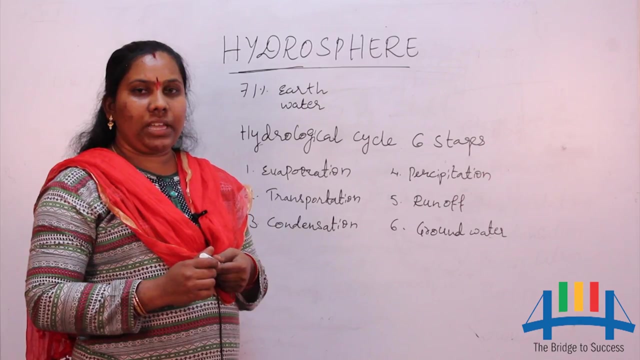 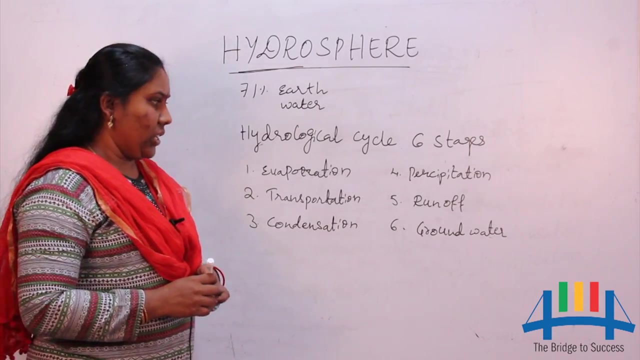 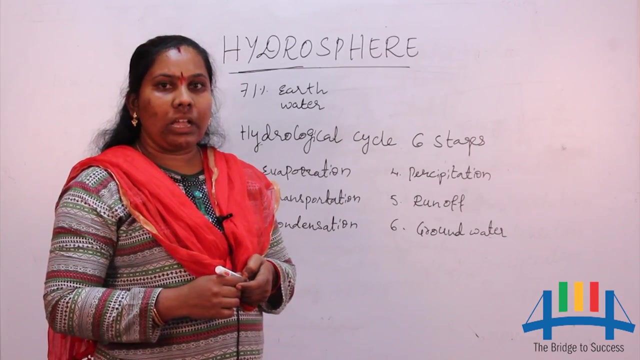 from the earth surface, it forms into the clouds. Those clouds move from the water surface area to the land surface area by upper air circulation or surface air circulation, For example the land and sea breezes. The third stage is condensation, where the clouds which interact with the atmosphere or air condense. 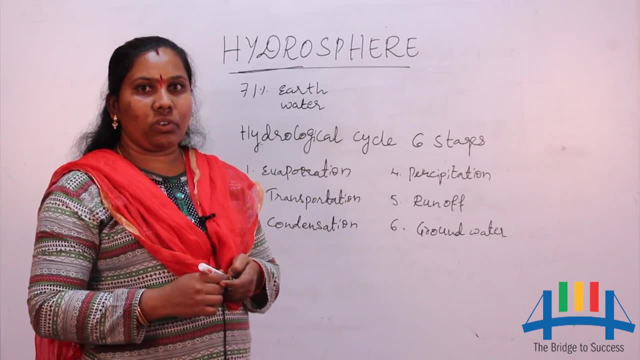 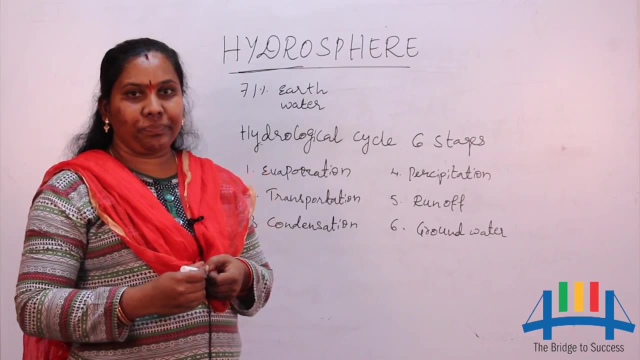 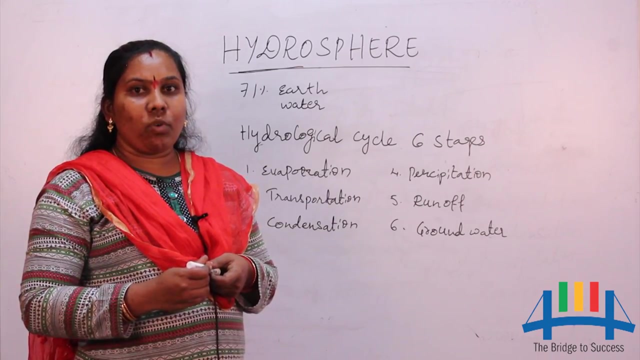 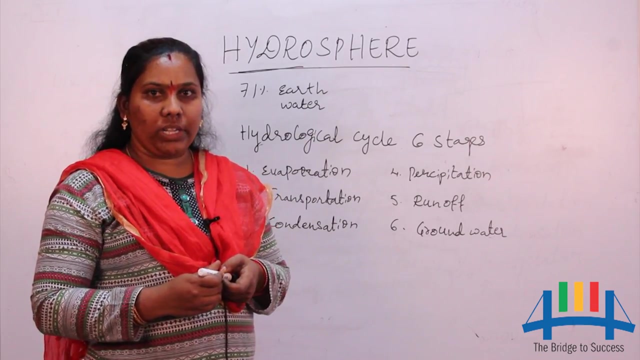 means cools down and forms into tiny droplets of water. For example, in a hot vessel, if you place a lid after a few minutes you can find the droplets of water. In the same way, when the water vapor goes down in the atmosphere, it forms like a tiny droplet of water. The fourth stage is precipitation. 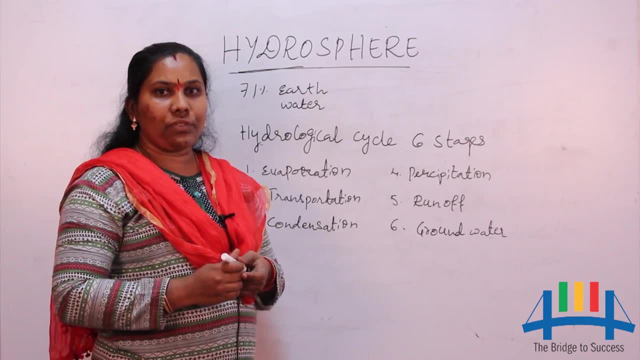 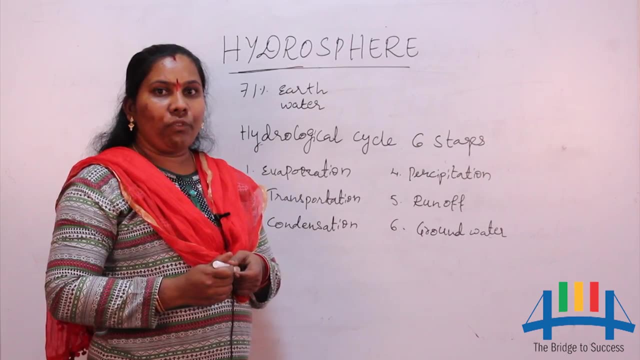 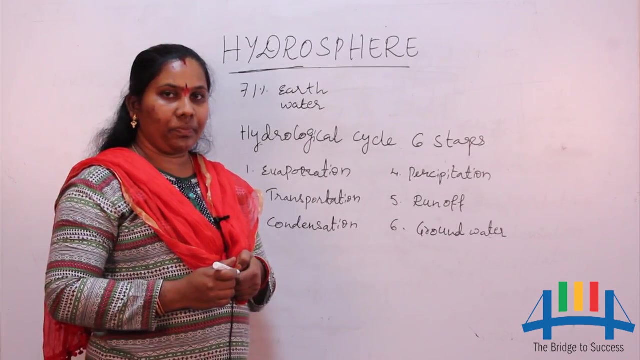 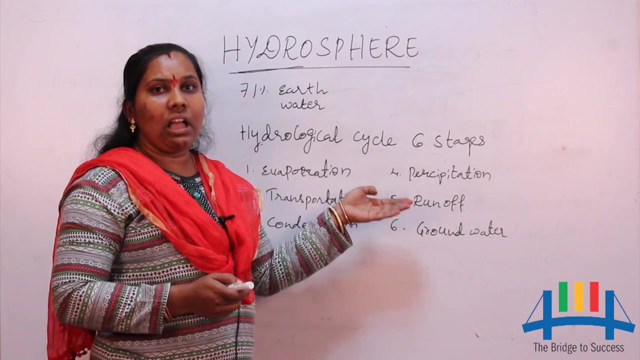 Those tiny droplets of water which are formed after the condensation is reaching the earth again, which is in the form of liquid stage. It can be like rain, slit or snow. The water which is reaching the earth, it is flowing from the hill area, that is, high level areas, to the low level areas that flow. 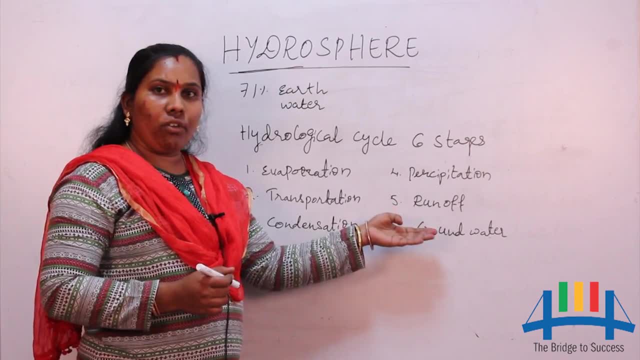 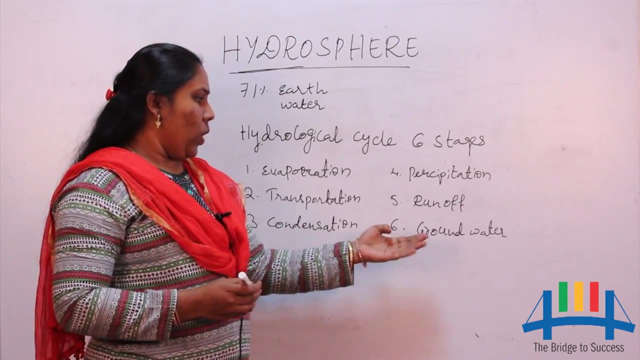 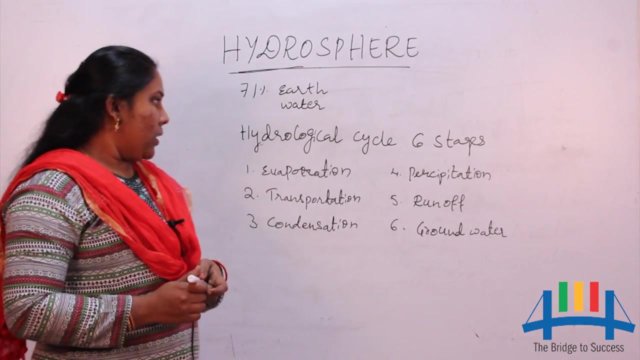 is nothing but the runoff. In the process of runoff, the water proclaims or pertains into the ground. The pertained water converts into the ground water, which is the sixth stage of the water cycle. Apart from this, you have the water sources, which we will discuss in the later class.